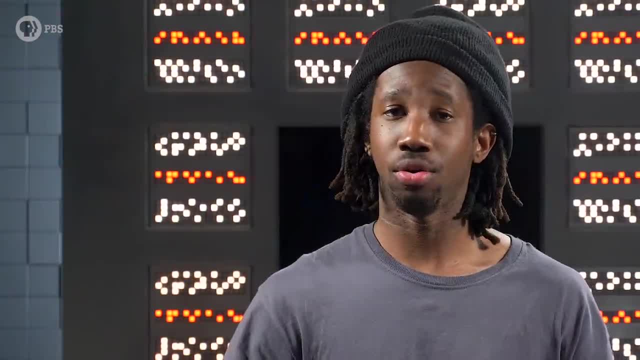 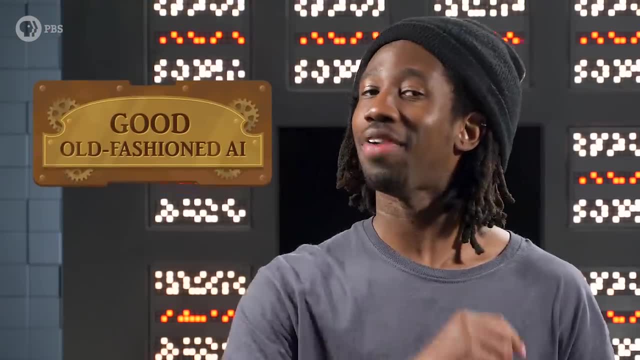 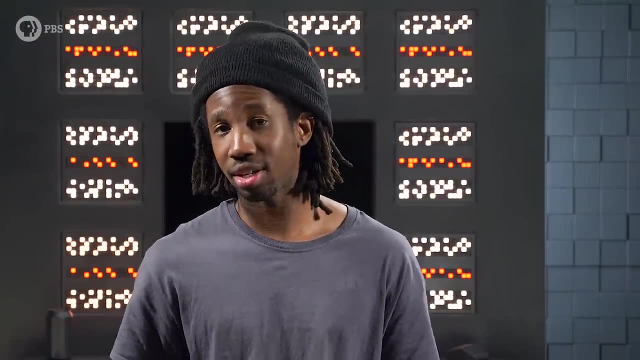 uses symbolic AI. Modern neural networks train a model on lots of data and predict answers using best guesses and probabilities, But symbolic AI- or good, old-fashioned AI, as it's sometimes called, is hugely different. Symbolic AI requires no training, no mass amounts of data and no guesswork. 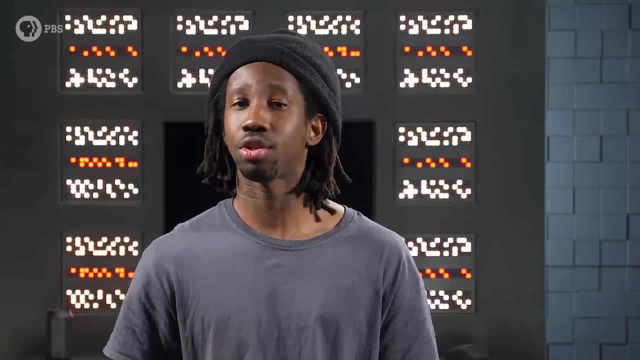 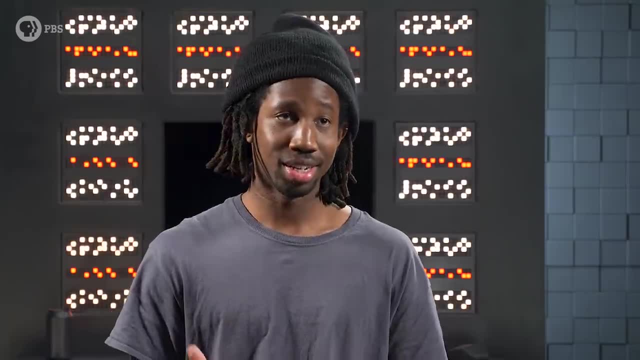 It represents problems using symbols and then uses logic to search for solutions. So all we have to do is represent the entire universe we care about as symbols in a computer- No big deal. To recap, logic is our problem-solving technique and symbols are how we're going to represent. 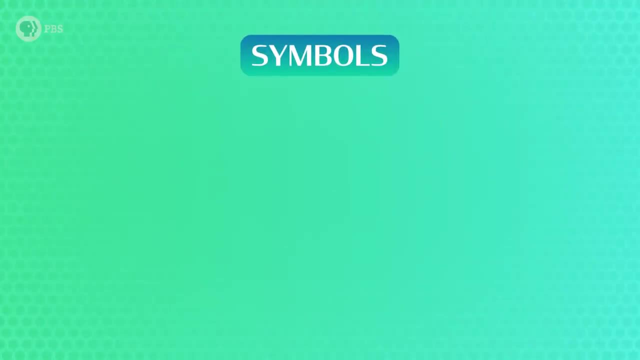 the problem. in a computer Now, symbols can be anything in the universe—numbers, letters, words, bagels, donuts, toasters, John Greenbots or jabrilles. One way we can visualize this is by writing symbols surrounded by parentheses, like donut. 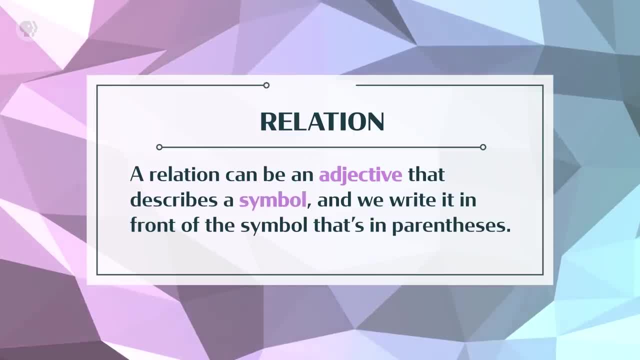 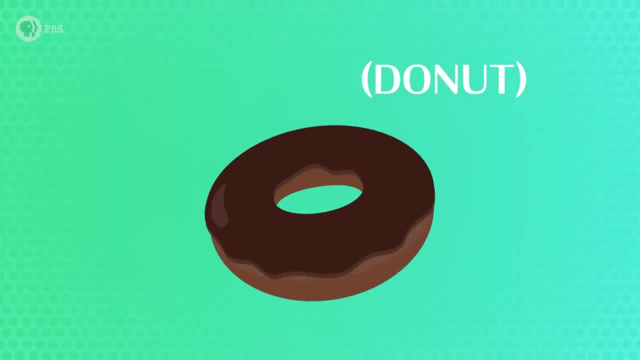 or jabrille. A relation can be an adjective that describes a symbol, and we write it in front of the symbol that's in parentheses. So, for example, if we wanted to represent a chocolate donut, we can write that as chocolate donut. 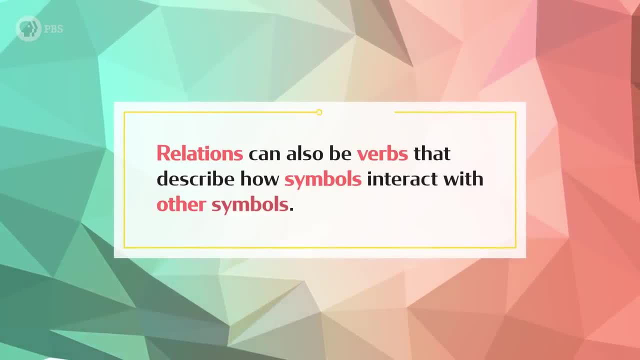 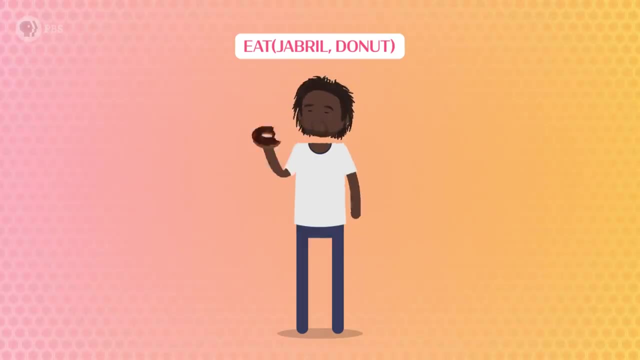 Relations can also be verbs that describe how symbols interact with other symbols. So, for example, I can eat a donut, which we will write as eat jabrille donut, Because the relation describes how one symbol is related to the other. 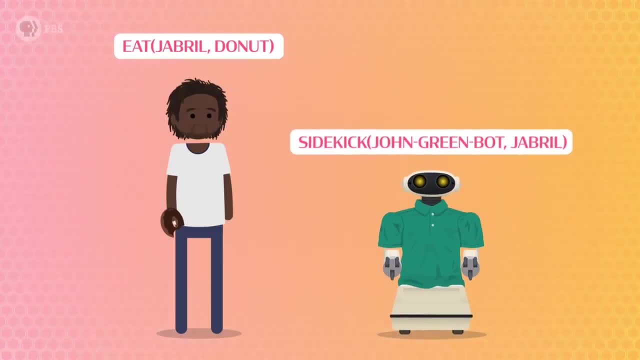 Or we can represent John Greenbot's relation to me using sidekick John Greenbot jabrille. A symbol can be a part of lots of relations, depending on what we want our AI system to do. So we can write others like: is John Greenbot robot or wears John Greenbot polo. 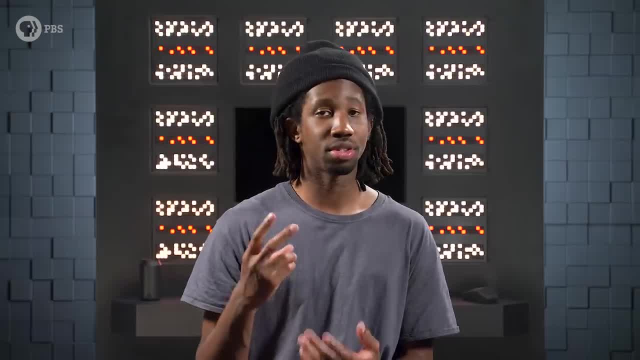 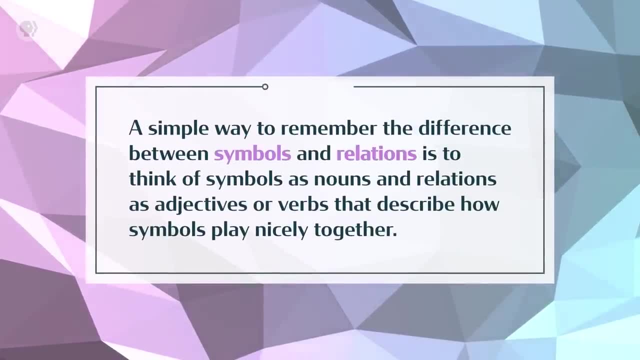 All of our examples in this video will include a max of two symbols for simplicity, but you can have any number of symbols described by one relation. A simple way to remember the difference between symbols and relations is by looking at the symbols as nouns and relations as adjectives or verbs that describe how symbols play nicely. 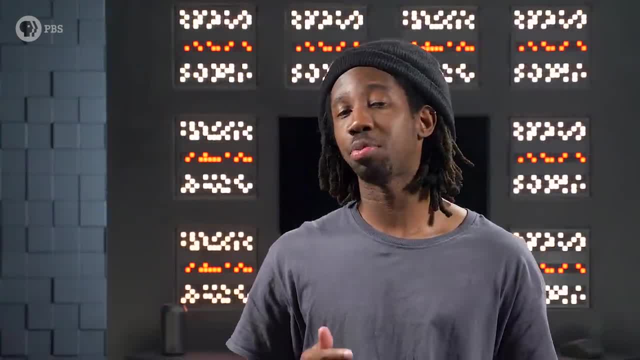 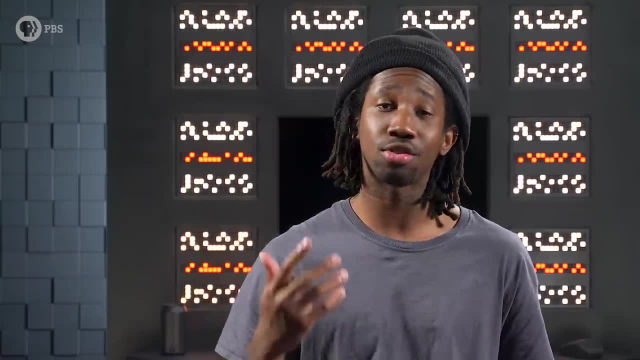 together. This way of thinking about symbols and their relations lets us capture pieces of our universe in a way that computers can understand, And then they can use their superior logic powers to help us solve problems. The collection of all true things about our universe is called a knowledge base. 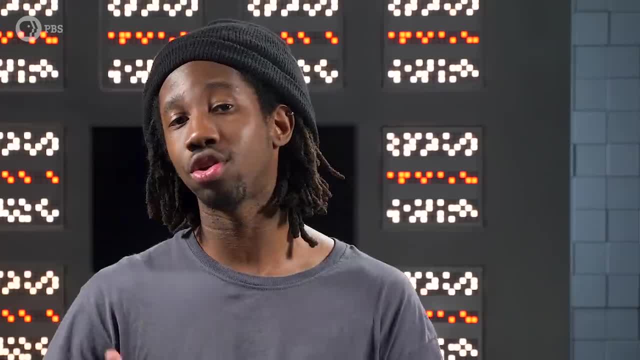 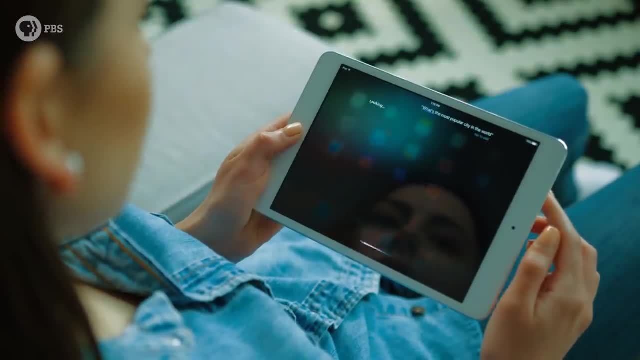 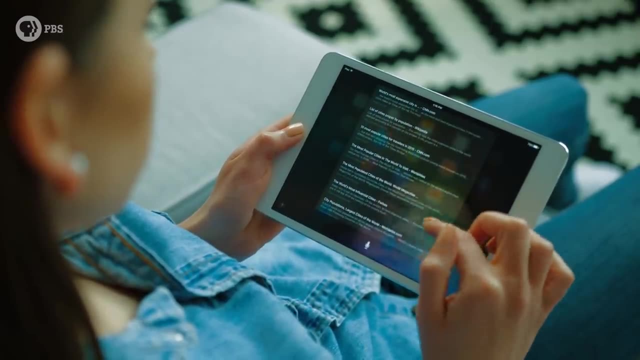 And we can use logic to carefully examine our knowledge bases in order to answer questions and to solve problems And discover new things with AI. This is basically how Siri works. Siri maintains a huge knowledge base of symbols, So when we ask her a question, she recognizes the nouns and verbs, turns the nouns into: 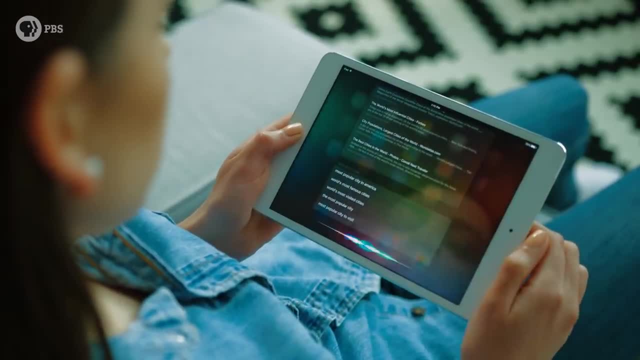 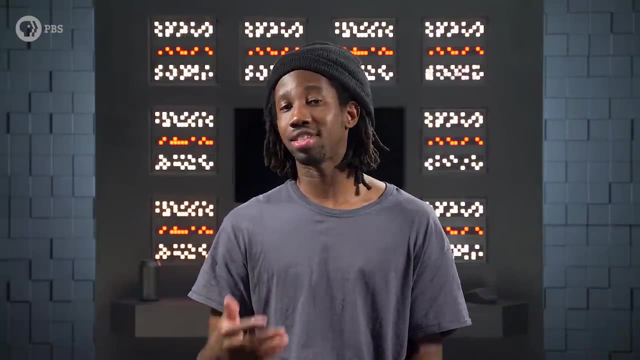 symbols and verbs into relations and then looks for them in the knowledge base. Let's try an example of converting a sentence into symbols and relations and then using logic to answer questions. Let's say John Greenbot drives a smelly old car. 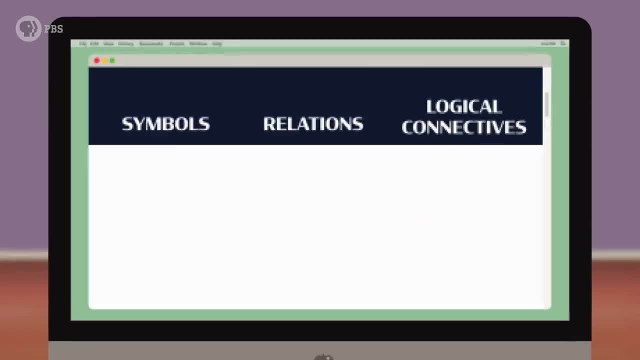 I could represent this statement in a simple way. Let's say: John Greenbot drives a smelly old car. I could represent this statement in a computer with symbols: John Greenbot and car, And then the relations drives smelly and old. Using logical connectives like AND and OR, we can combine these symbols to make sentences. 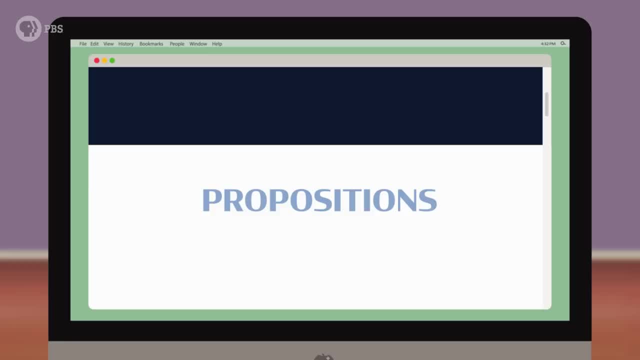 called propositions, And then we can use a computer to figure out whether these propositions are true or not, using the rules of propositional logic in a tool called a truth table. Propositional logic is basically a fancy name for Boolean logic, which we covered in episode. 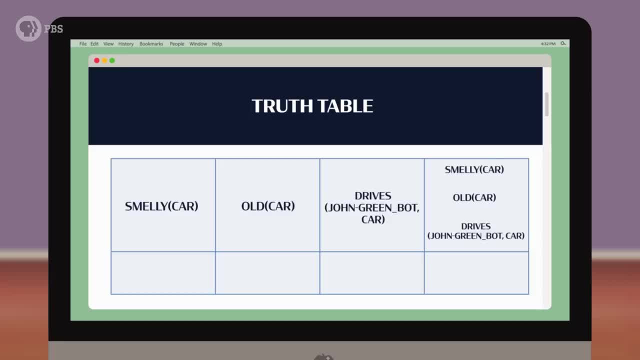 3 of Crash Course, Computer, And the truth table helps us decide what's true and what's not. So in this example, if the car is actually smelly and actually old and if John Greenbot actually drives the car, then the proposition: smelly car AND old car AND John Greenbot drives. 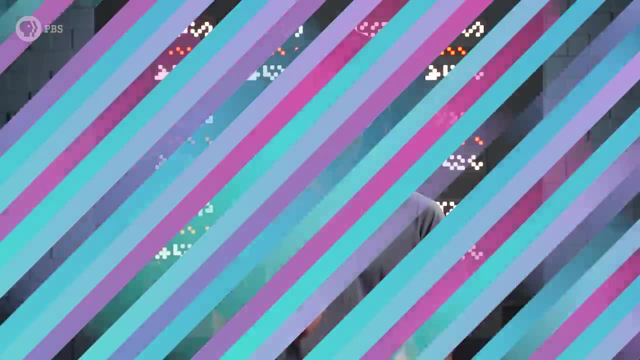 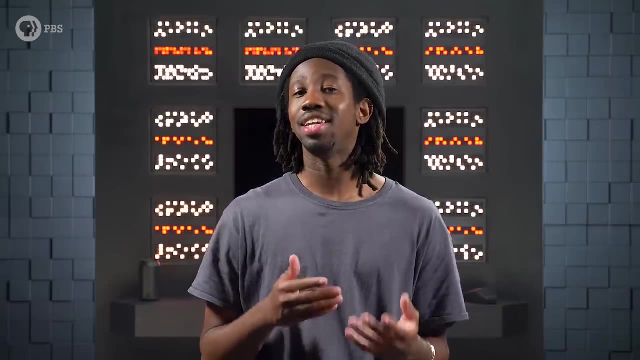 the car is true. We can understand that sort of logic with our brains. If all three things are true, then the whole proposition is true, But for an AI to understand that it needs to use some math. So let's try this. 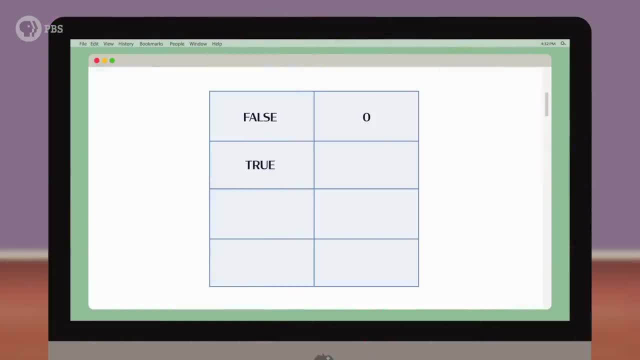 If we have a computer, we can think of a false relation as 0 and true relations as any number that's not 0. We can also think of ANDs as multiplication and ORs as addition. But let's look at what's happening to the math if the car is not actually old. 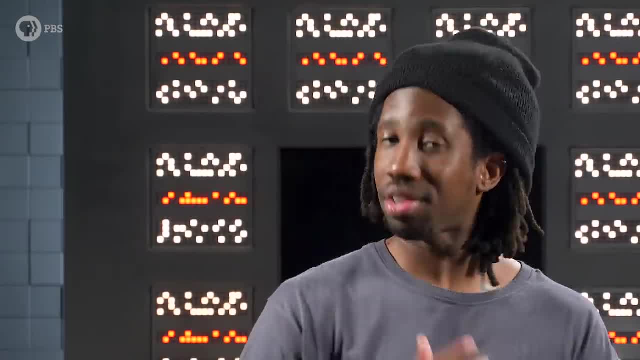 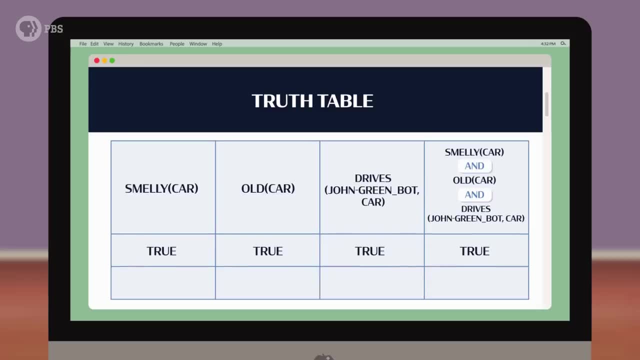 Again, our brains might be able to jump to the conclusion: If one of the three things isn't true, then the whole proposition must be false. But to do the math like an AI would, we can translate this proposition as true times, false times, true. 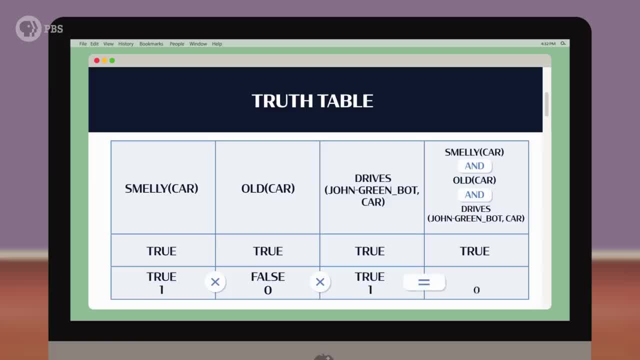 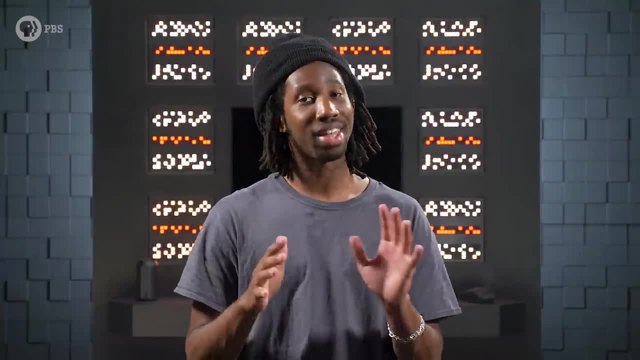 Which is 1 times 0 times 1.. That equals 0, which means the whole proposition is false. So that's the basics of how to solve propositions that involve AND. But what if we want to know if John Greenbot drives a car AND that the car is either smelly, 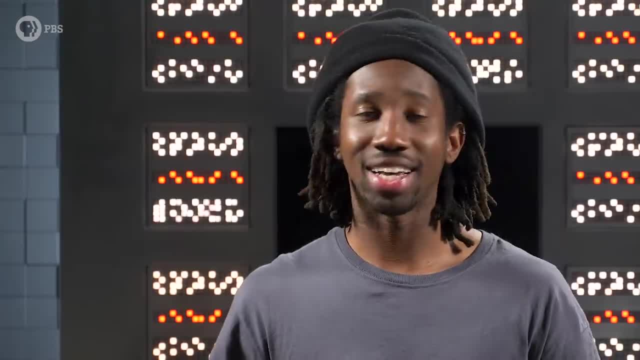 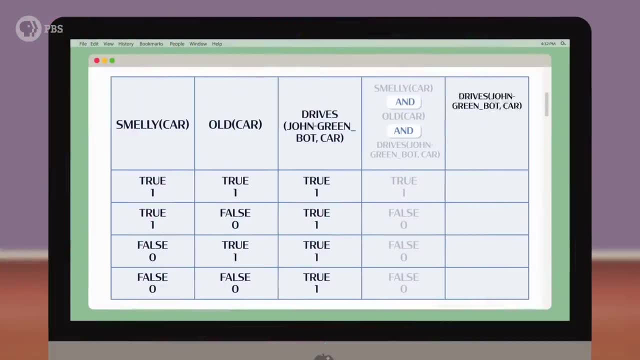 OR old, Like I mentioned earlier, OR can be translated as addition. So, using our math rules, we can fill out this new, bigger truth table. The proposition we're dealing with now is smelly car OR old car And John Greenbot drives the car. 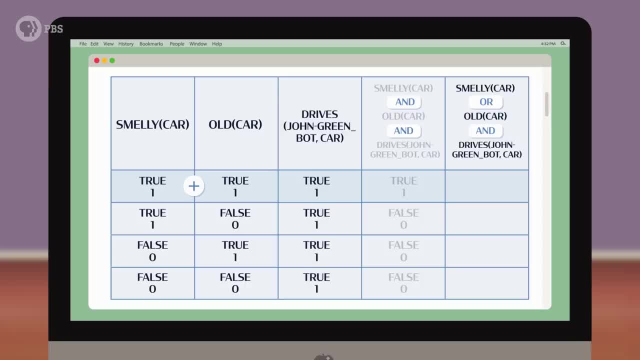 For the first row. this translates as true plus true. Then that result times true, which we calculate as 1 plus 1 times 1.. That equals 2 times 1,, which is 2, which means the whole proposition is true. 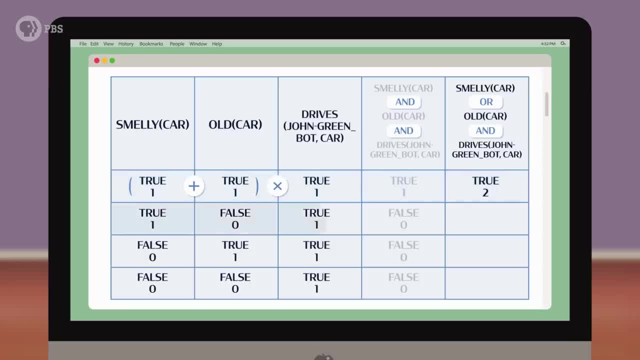 Remember: any answer that isn't 0 is true. The second row translates as true plus false. Then that result times true, which we calculate as 1 plus 0. That's true times one. That equals one times one, which is one, which means the whole proposition. 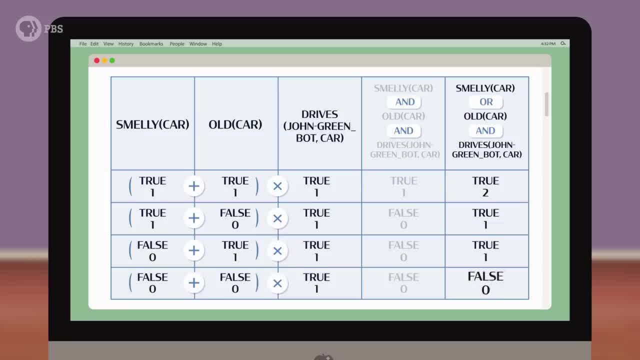 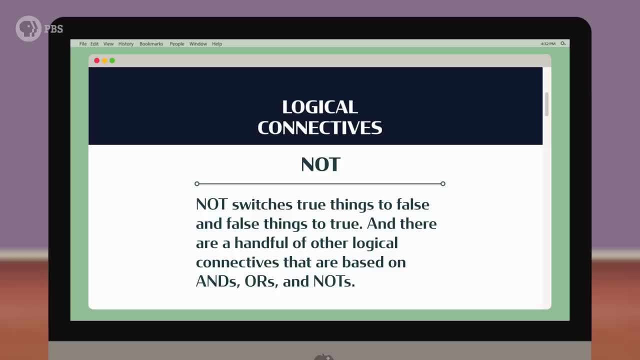 is true again, And we can fill out the rest of the truth table the same way. Another logical connective besides AND and OR is NOT, which switches true things to false and false things to true, And there are a handful of other logical connectives that 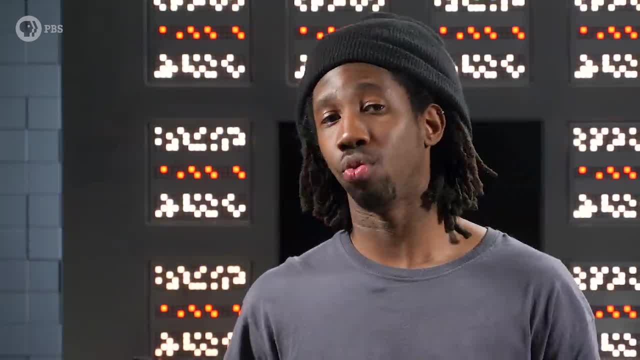 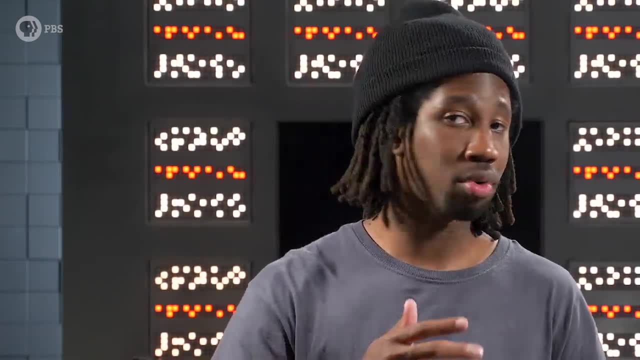 are based on ANDs, ORs and NOTs. One of the most important ones is called implication, which connects two different propositions. Basically, what it means is that if the left proposition is true, then the right proposition must also be true. 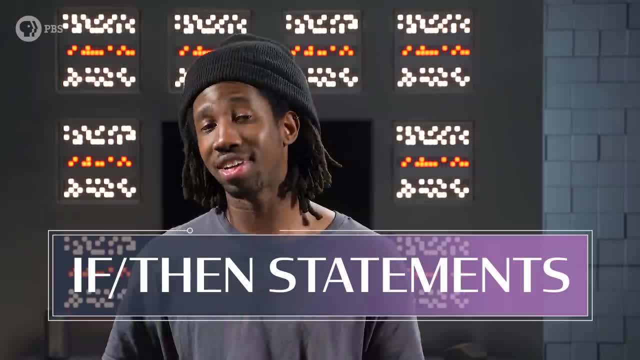 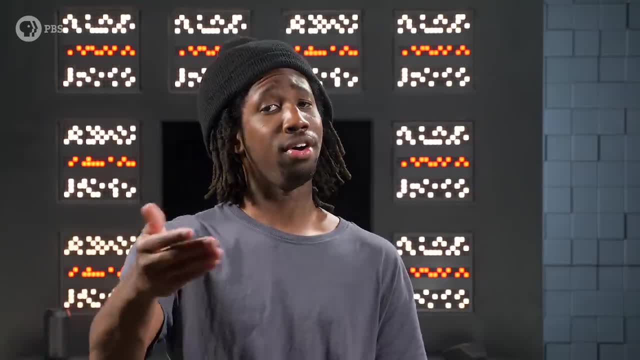 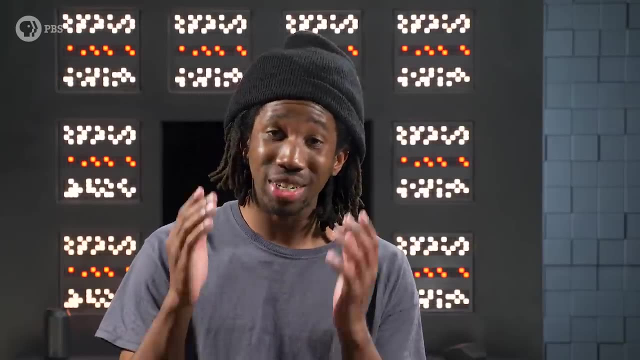 Implications are also called If-then statements. We make thousands of tiny if-then decisions every hour, Like, for example, If tired, then take nap, Or If hungry, then eat snacks, And modern symbolic AI systems can simulate billions of if-then statements every second. 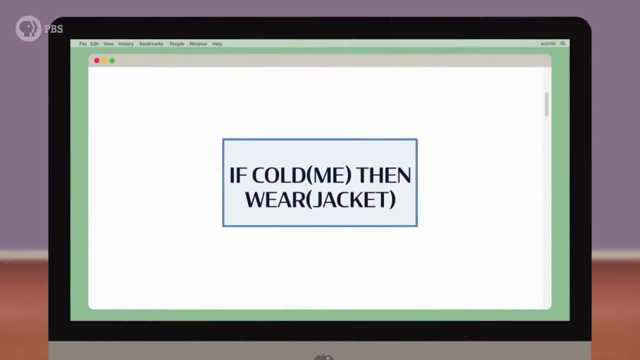 To understand implications. how about we use a new example: If I'm cold, then I wear a jacket. This is saying that if I'm definitely cold, then I must be wearing my jacket, But if I'm not cold, I can wear whatever I want. 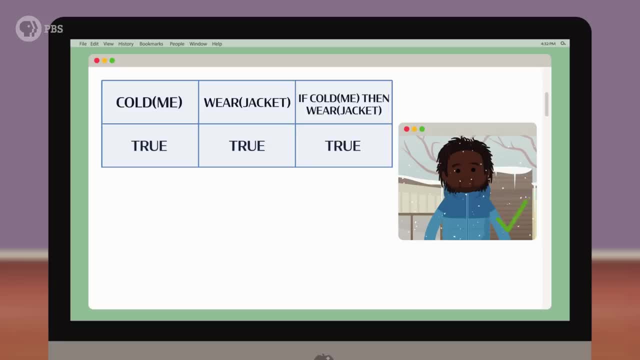 So if cold is true and jacket is true, both sides of the implication are true. Even if I'm not cold and I wear my jacket, then the statement still holds up. Same if I'm not cold and I decide to not wear my jacket. 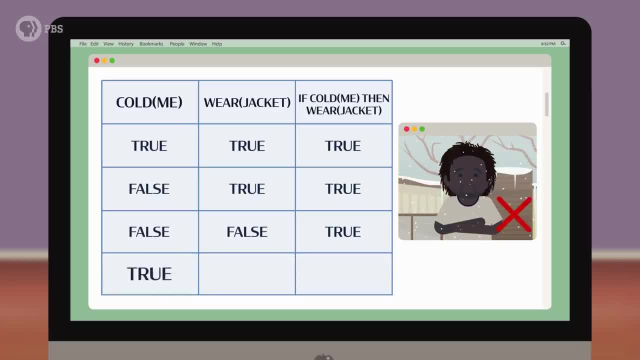 I can do whatever I want, since I'm not cold. But if I am cold and I decide not to wear my jacket, then the statement no longer works. The implication is false. Simply put, an implication is true if the then side is true or the if side is false. 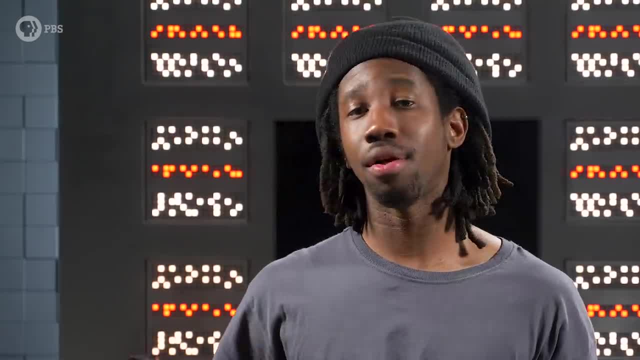 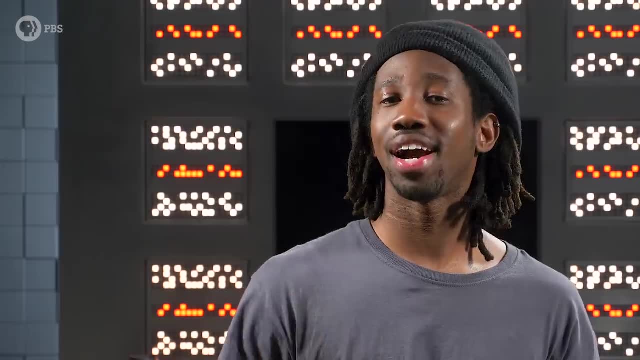 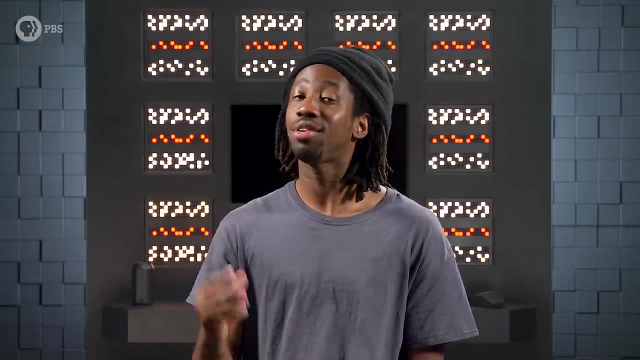 Using the basic rules of propositional logic, we can start building a knowledge base of all the propositions that are true about our universe. After that knowledge base is built, we can use symbolic AI to answer questions and discover new things. So, for example, if I were to help John Greenblatt start building a knowledge base, I'd tell 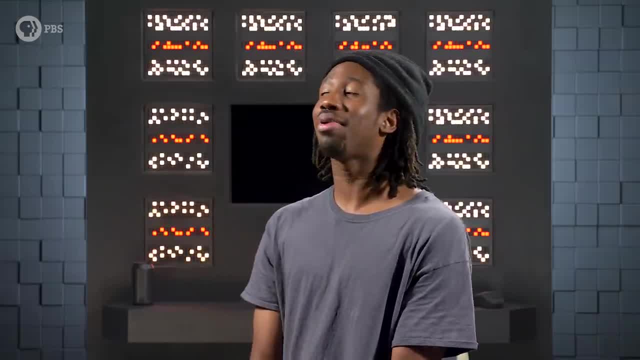 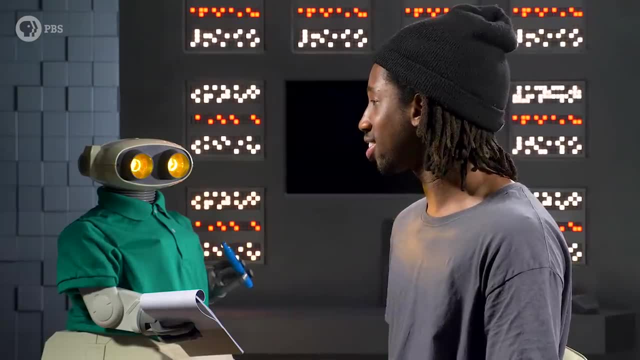 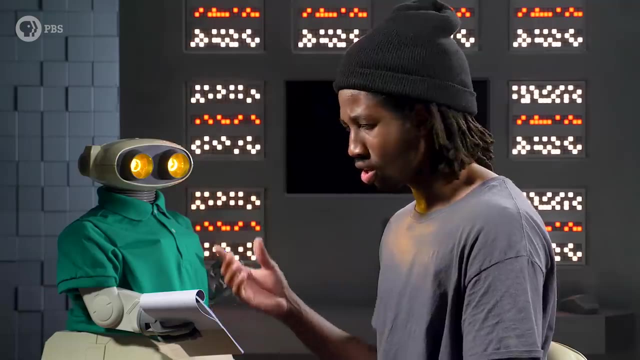 him a bunch of true propositions. Oh, John Greenblatt. All right, you ready, John Greenblatt. So Jabril is person, John Greenblatt is machine, Car is machine, Car is old, Car is smelly. John Greenblatt is not person. 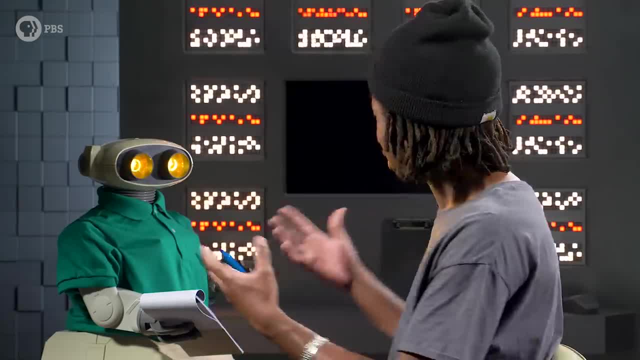 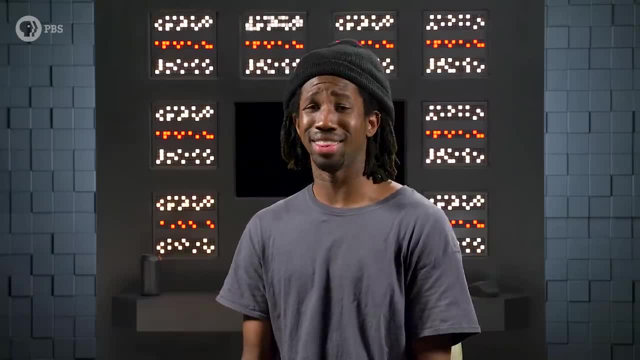 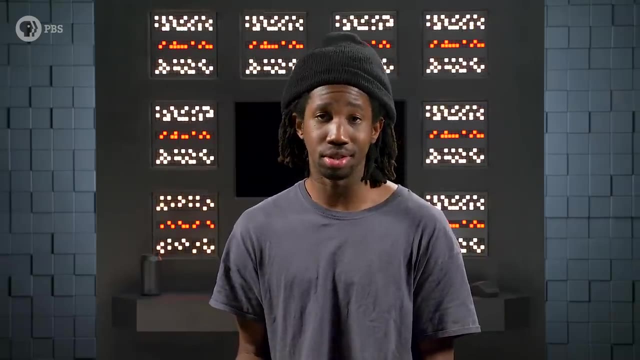 Jabril isn't machine, Toaster is machine. You getting all this, John Greenblatt? Clearly, at this pace, John Greenblatt would never be able to build a knowledge base with all the possible relations and symbols that exist in the universe. 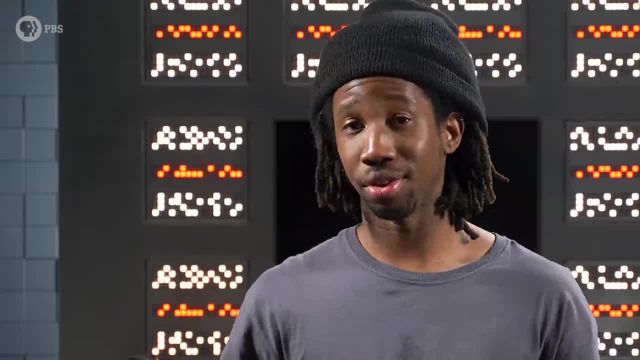 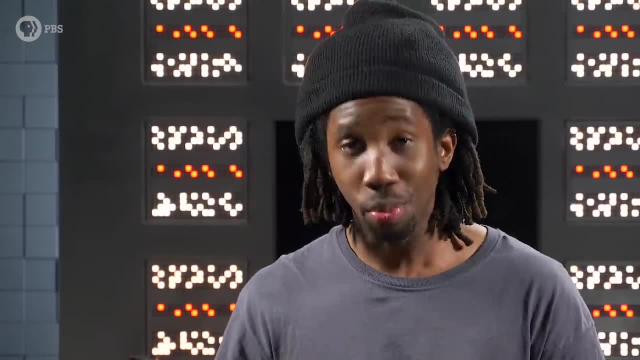 There are just too many. Fortunately, computers are really good at solving logic problems, So if we populate a knowledge base with some propositions, then we can use a program to find new propositions that fit with the logic of the knowledge base without humans telling it every single one. 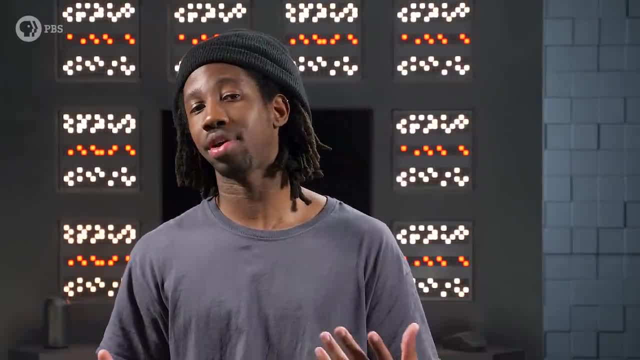 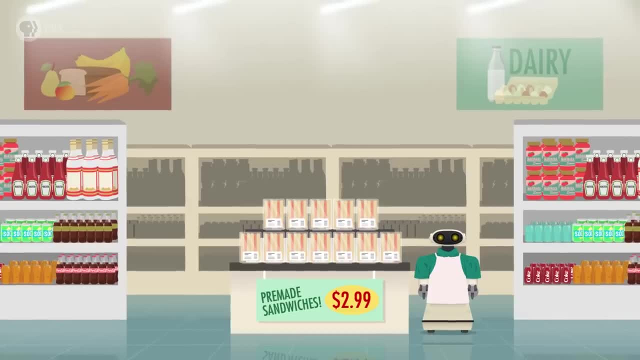 So if we populate a knowledge base with some propositions, then we can use a program to find new propositions that fit with the logic of the knowledge base without humans telling it every single one. This is called inference. For example, the knowledge base of a grocery store might have a proposition that sandwich. 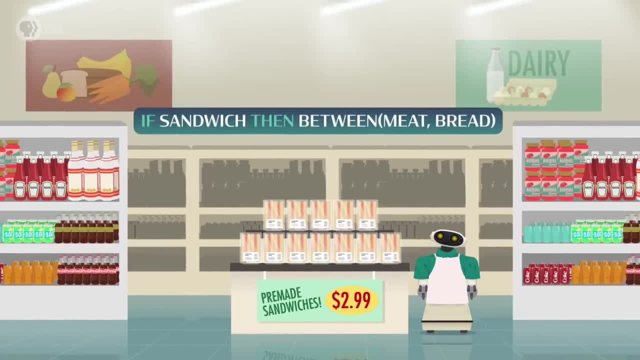 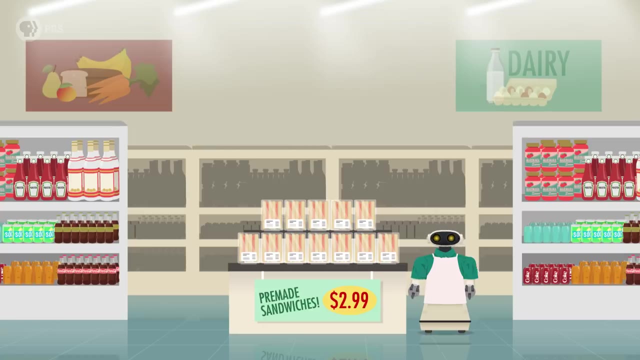 implies between meat bread or if sandwich, then between meat bread. Meat and bread are the symbols and between is the relation that defines them. So, basically, this proposition is defining a sandwich as a symbol with meat between bread. Simple enough. There are other rules in the grocery knowledge base. 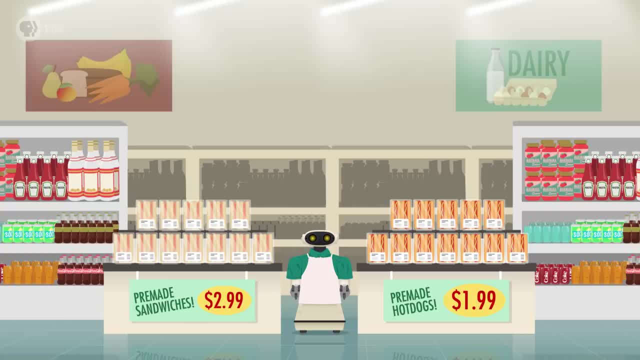 Like, for example, a hot dog, also implies between meat bread, or if hot dog, then between meat bread. Now, if the grocery store is having a sale on sandwiches, should the hot dogs also be on sale? Well, with inference, the grocery store AI system can apply the following logic: 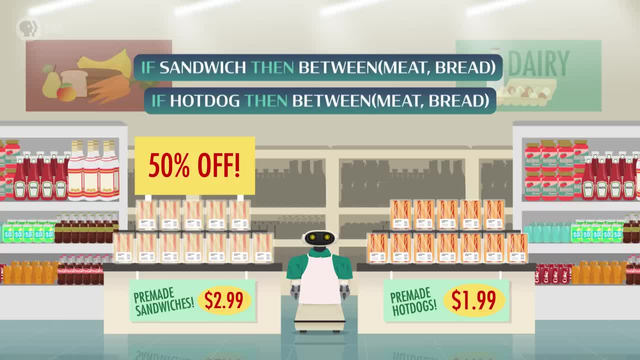 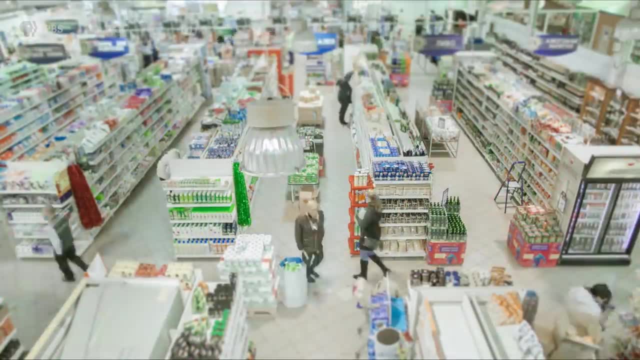 Because sandwiches and hot dogs are both symbols that imply meat between bread, then hot dogs are inferred to be sandwiches and the discount applies. Over the years, we've created knowledge bases for grocery stores, banks, insurance companies and other industries to make important decisions. 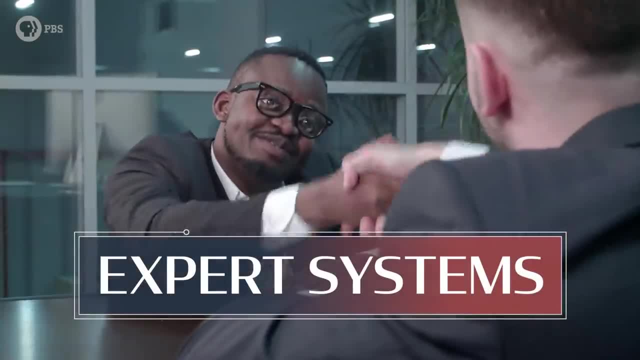 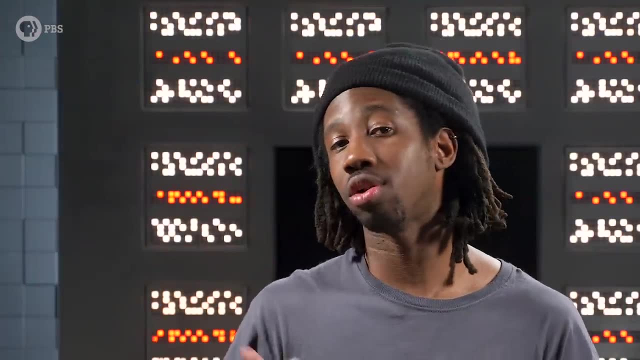 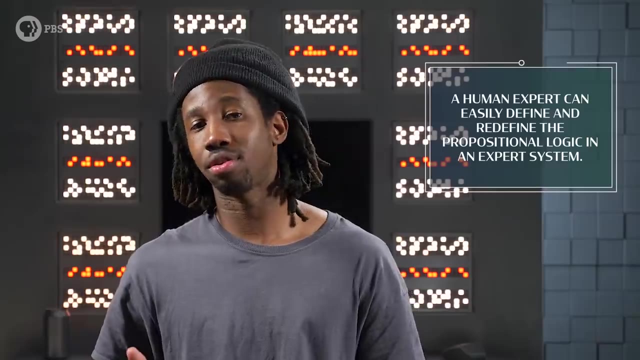 These AI systems are called expert systems because they basically replace an expert like an insurance agent or a loan officer. Symbolic AI expert systems have some advantages over other types of AI that we talked about, like neural networks. First, a human expert can easily define and redefine the propositional logic in an expert 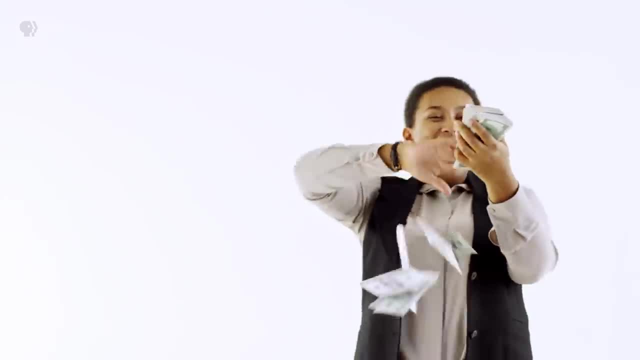 system: If a bank wants to give out more loans, If it can give out more bonds, Then it does, Then it doesn't. Then it does, Then it doesn't, Then it doesn't. For example, they can change the propositions involving credit score or account balance. 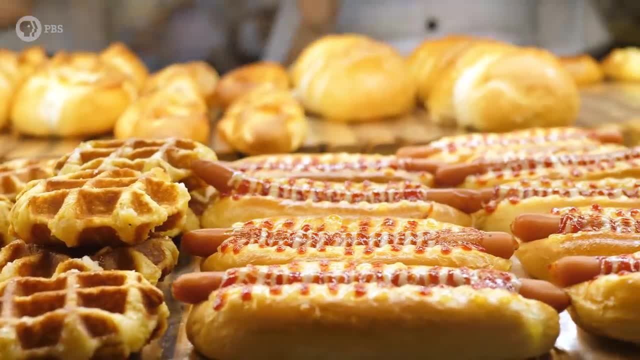 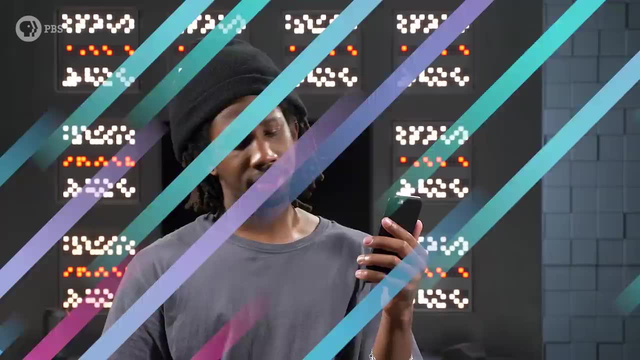 rules in their AI knowledge base. If a grocery store decides they don't want to discount hot dogs during the sandwich sale, then they might redefine what it means to be a sandwich or a hot dog. Hey, Siri, is a hot dog a sandwich? 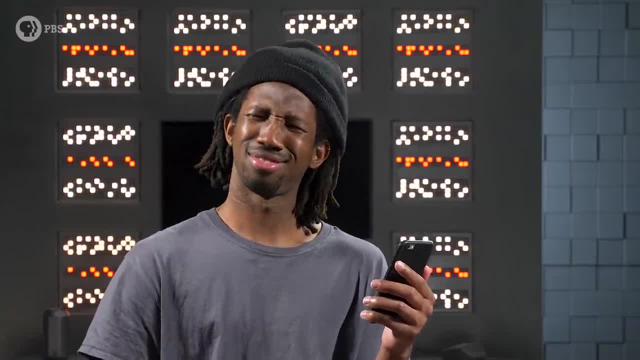 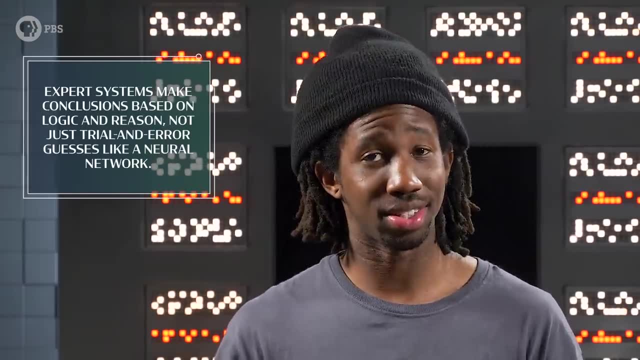 Of course not, Jabril. do not waste my time with foolish questions. Second, expert systems can make conclusions based on logic and reason, not just trial and error guesses like a neural network. And third, an expert system can explain its decisions by showing which parts were evaluated. 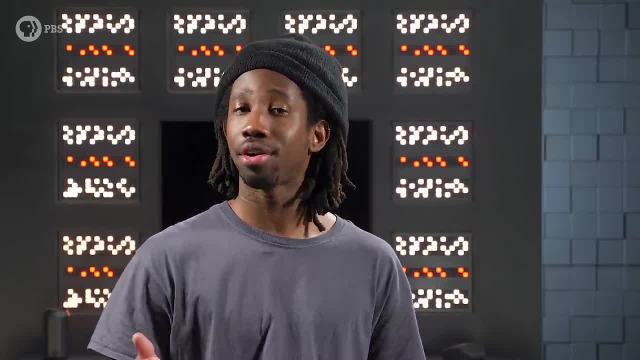 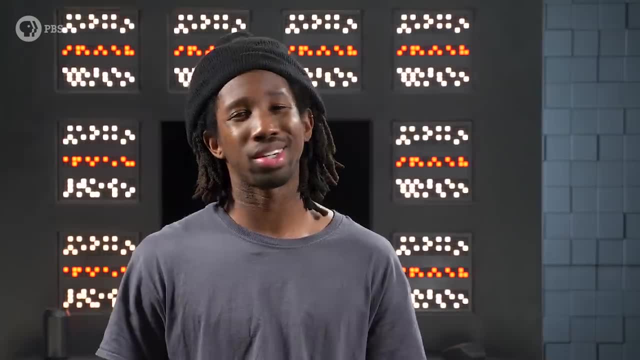 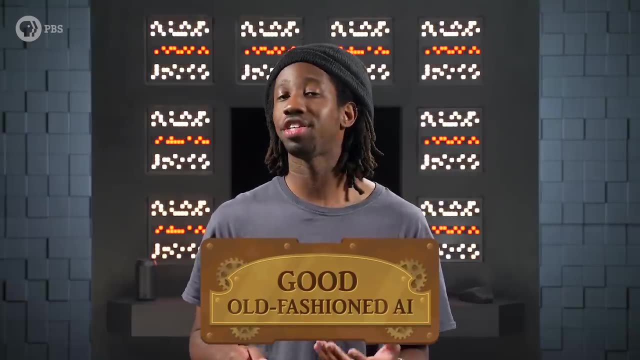 as true or false. A symbolic AI can show a doctor why it chose one diagnosis over another, or explain why an auto loan was denied. The hidden layers of a neural network just can't do that, At least not yet. This so-called good old fashioned AI has been really helpful in situations where the rules. 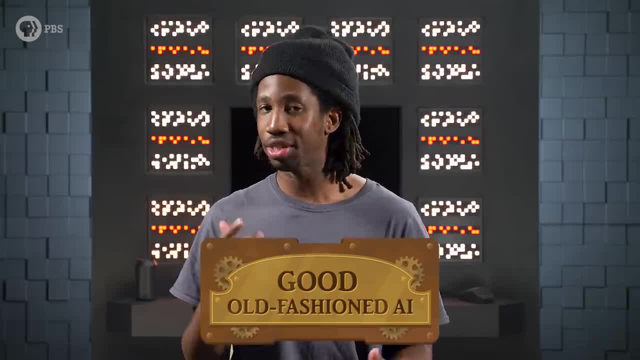 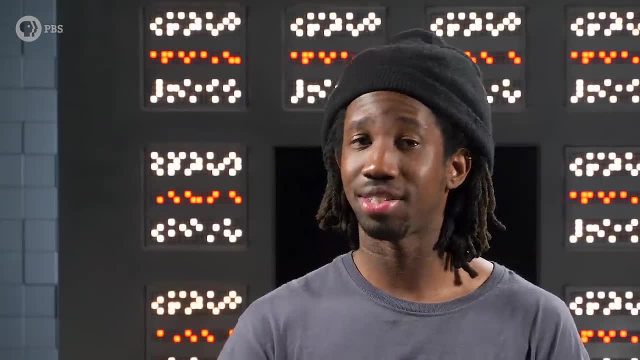 are obvious and can be explicitly entered as symbols into a knowledge base, But this isn't always as easy as it sounds. How would you describe a hand-drawn number 2 as a symbol in a numbered knowledge base? It's not that easy.